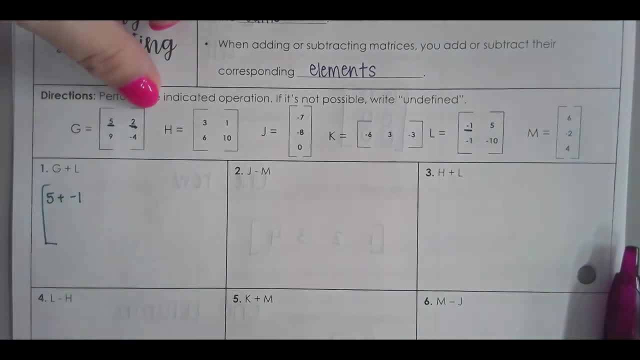 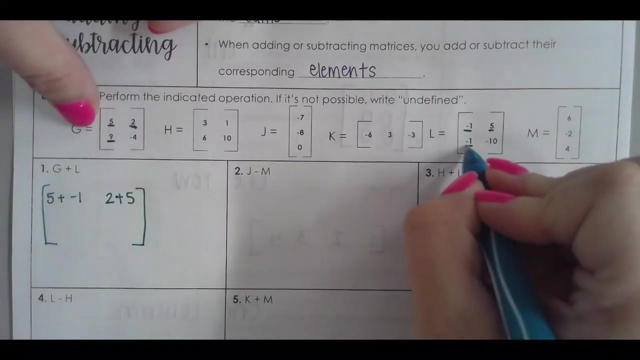 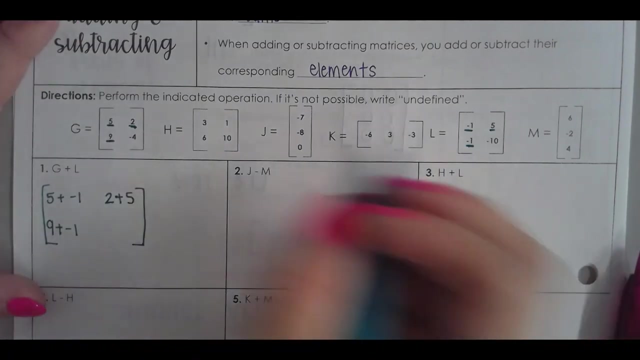 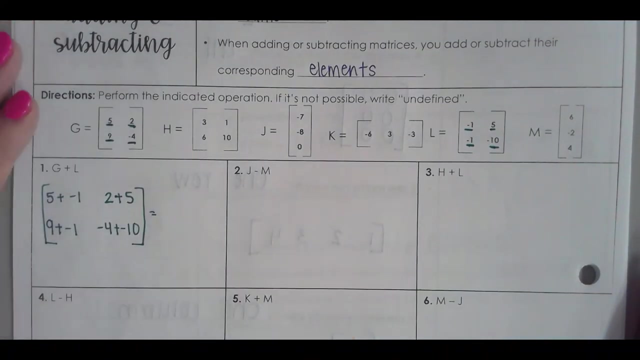 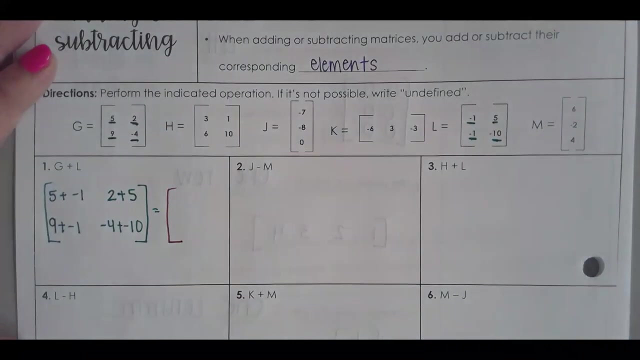 We're going to add 2 and 5.. We'll add 9 and negative 1.. Those are both second row, first column, And negative 4 and negative 10.. What are they? Negative 10.. Negative 11.. 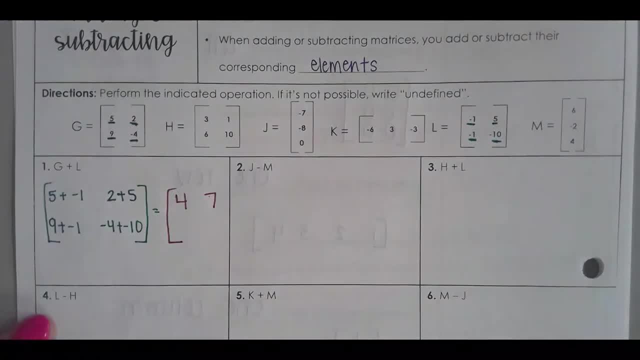 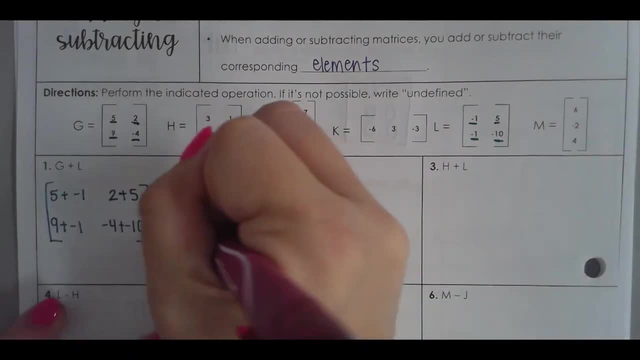 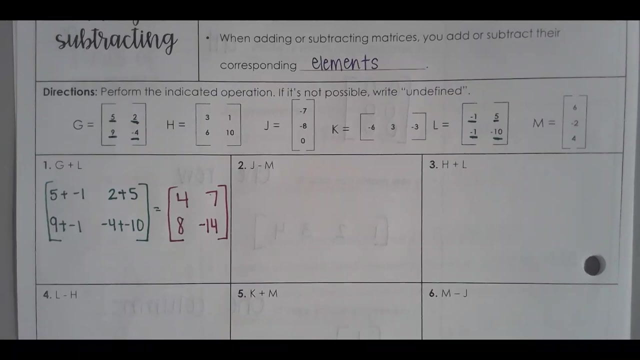 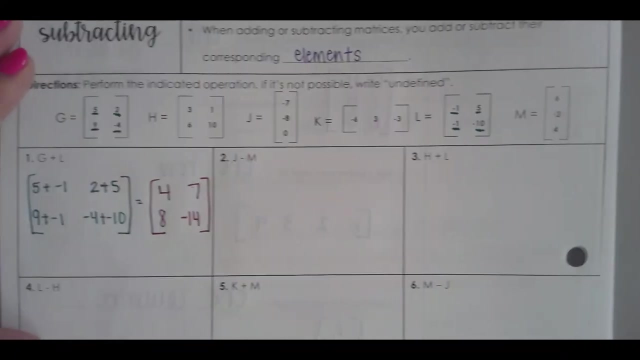 Add the 2 and negative 6.. Add the 2's. Add the 4.. Add the 6.. Line your sum 0 and negative: 2, negative 6.. Add the 2's: J minus M. 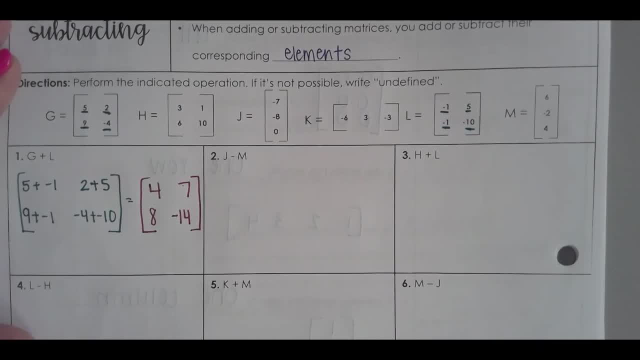 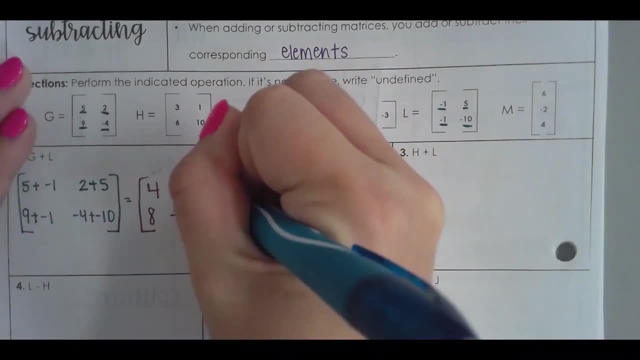 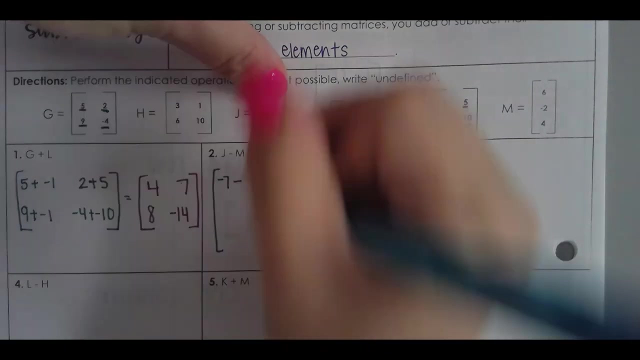 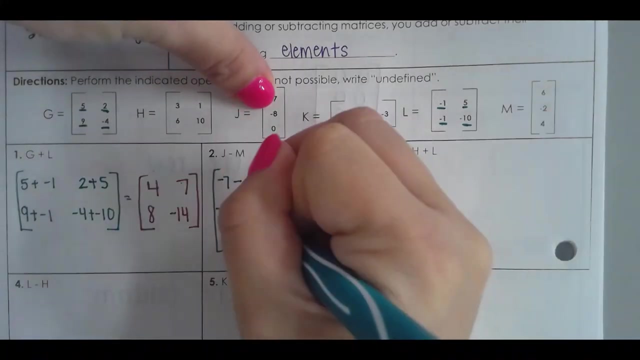 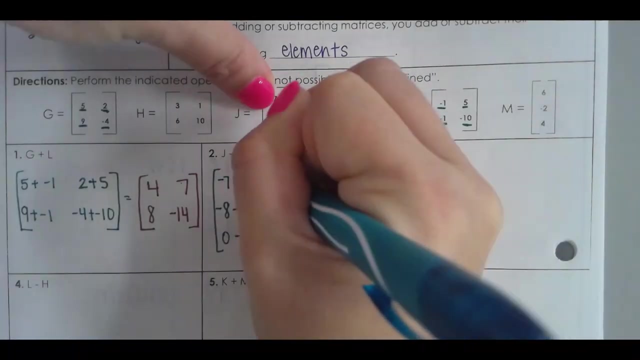 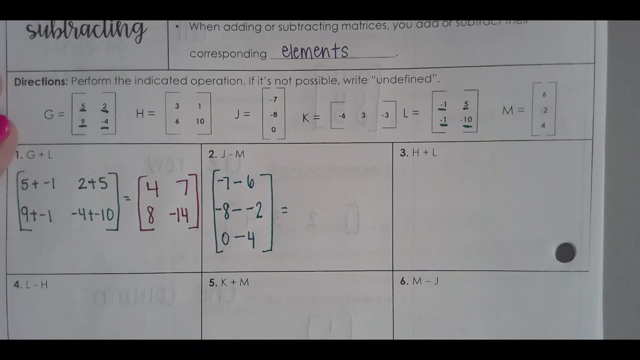 Can we do it? No, Yeah, you can. J and M are the same dimensions, All right, So it's minus negative 7 minus 6, negative 8 minus negative 2, and 0 minus 4.. Negative 7 minus 6 is what. 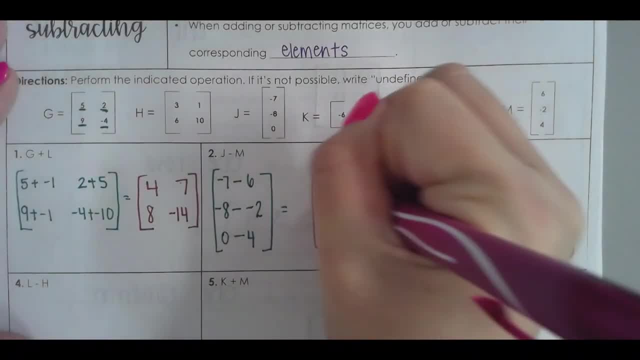 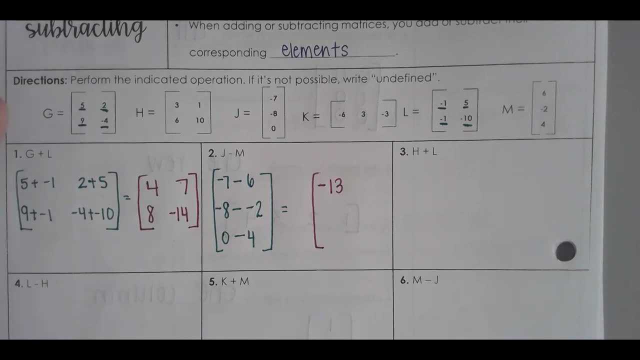 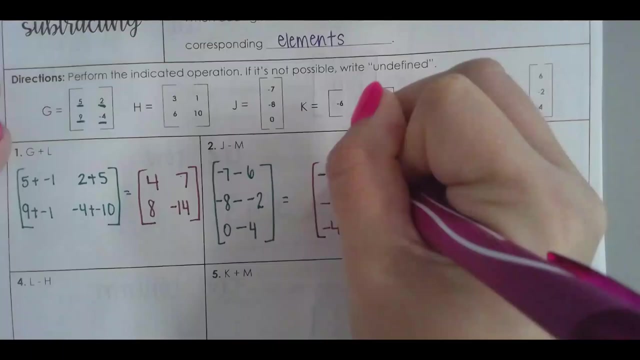 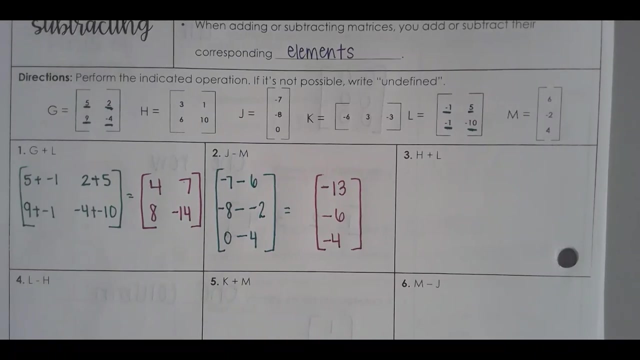 Negative 13. Good Negative: 8 minus negative: 2. Yep negative: 6. And 0 minus 4, negative 4.. All right, Any questions? All right, Number 3. A plus L. Can we do it? 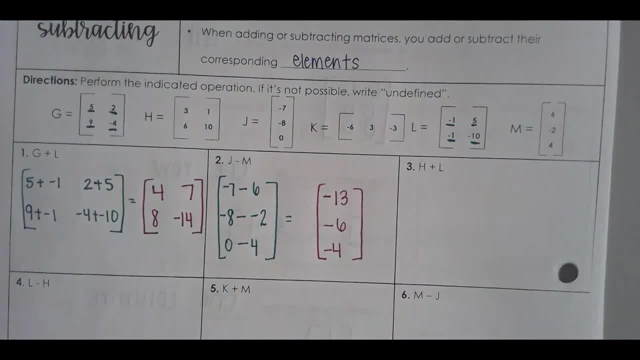 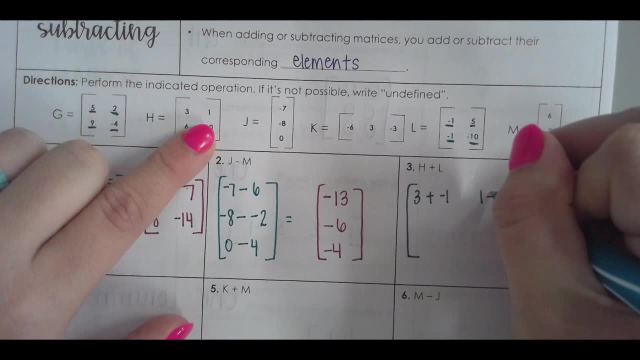 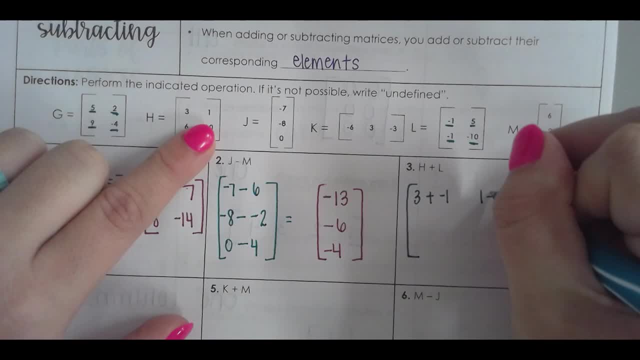 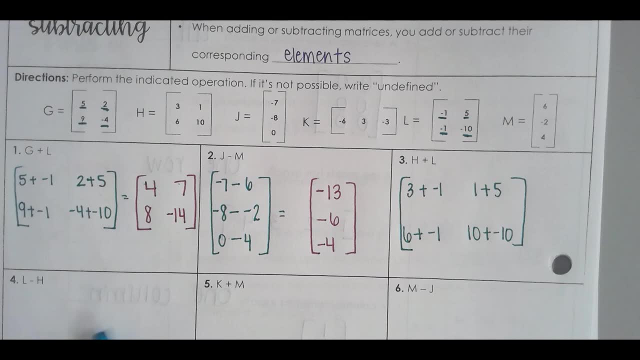 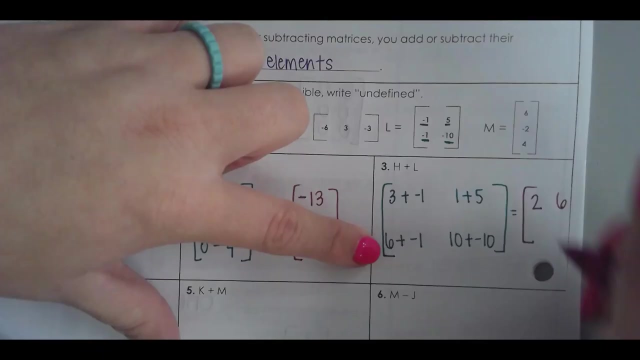 1. And 10 plus negative. 1 is 2.. 1 plus 5 is 9.. 10 plus negative 10.. Alright, I want you to do 4,, 5, and 6. If it can't be done, you can just. 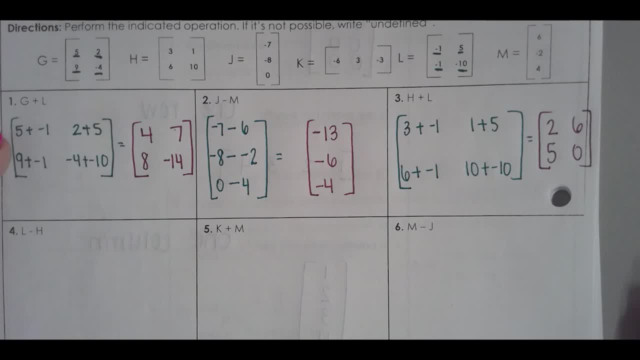 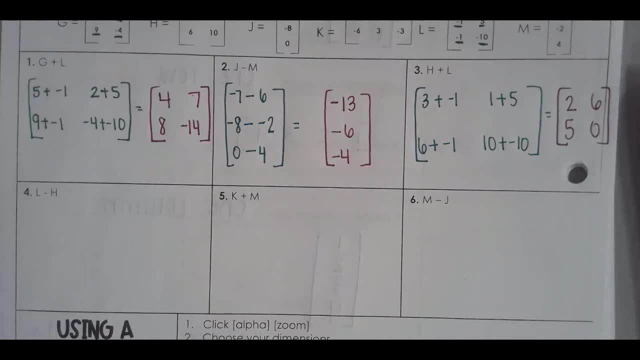 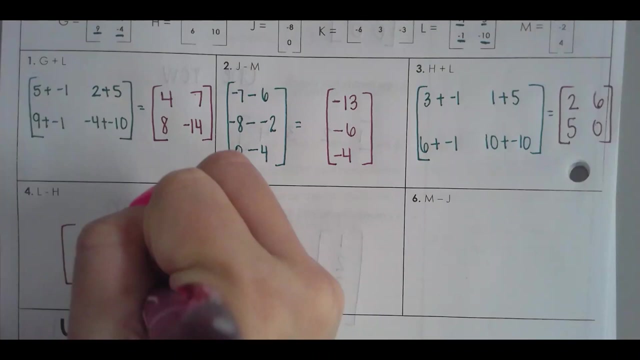 where possible? Alright, let's go over these Number 4.. Livia, was number 4 possible? What are the dimensions of your answer in number 4?? Kiera, can you tell me the numbers that you got in number 4?? 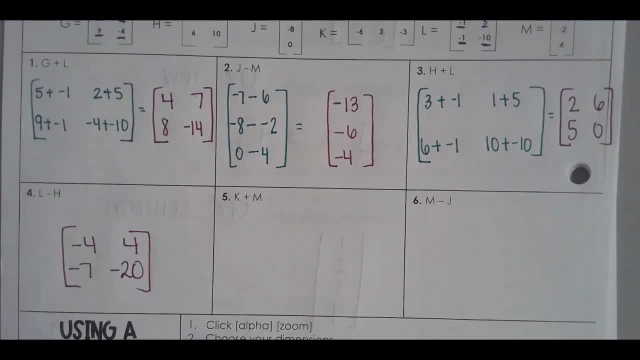 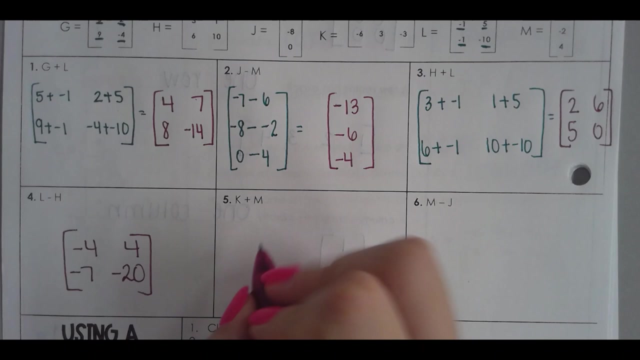 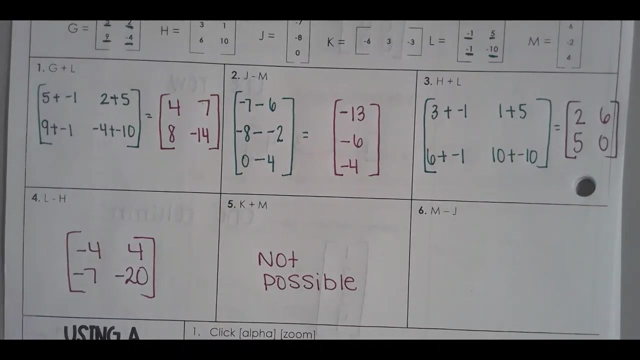 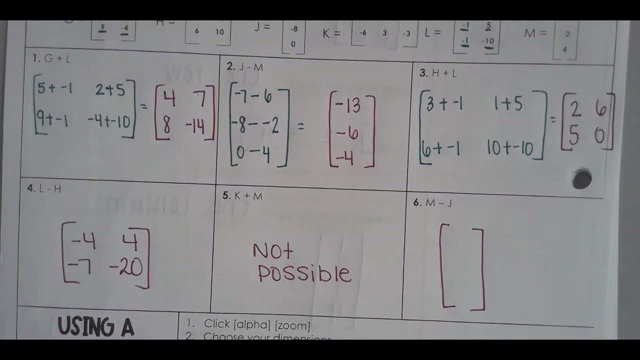 4,, negative 7, and negative 20.. What are the dimensions of your answer in joke 2?? Number six, Laren, was it possible? This would be a three, Three by one. What numbers are in the matrix? 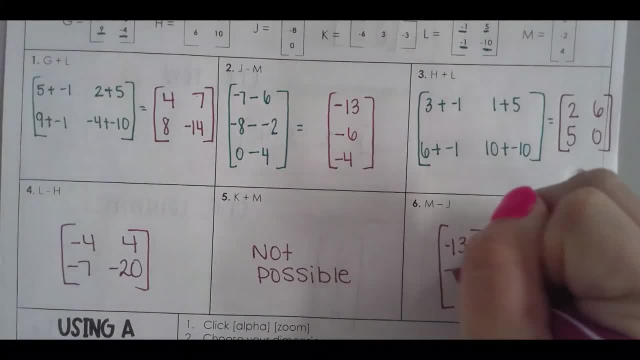 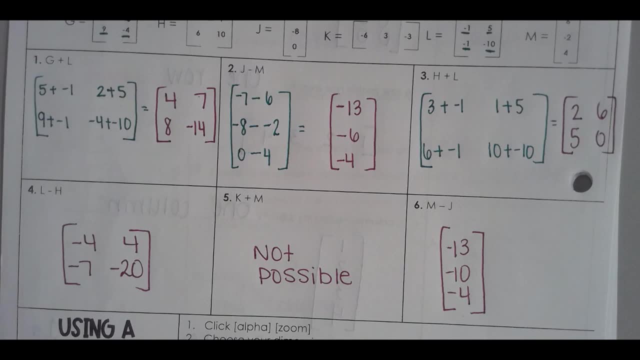 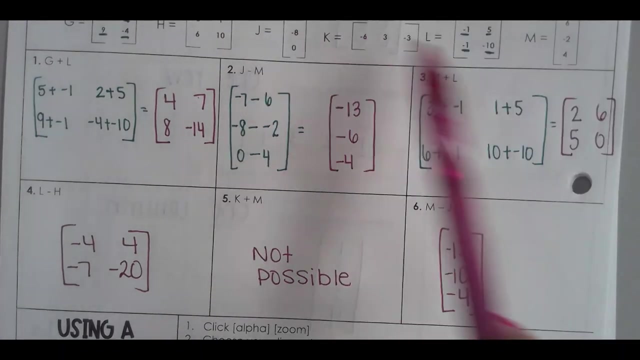 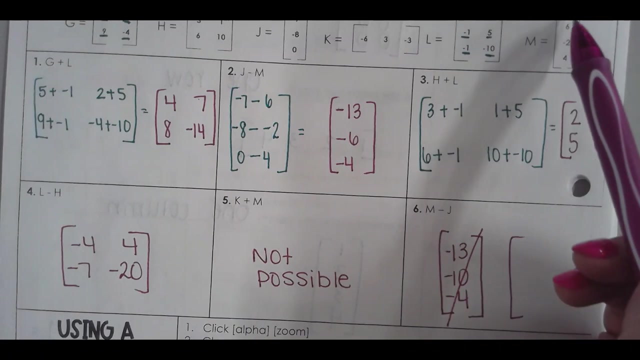 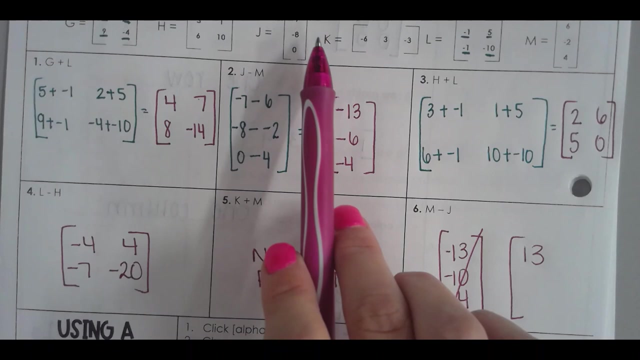 Negative 13,, negative 10, and negative 4.. Does that look right? Y'all disagree. I got 13,, 16, and 4.. You probably did J minus M. All right, So M minus J, J, 6 minus negative, 7 is positive 8.. 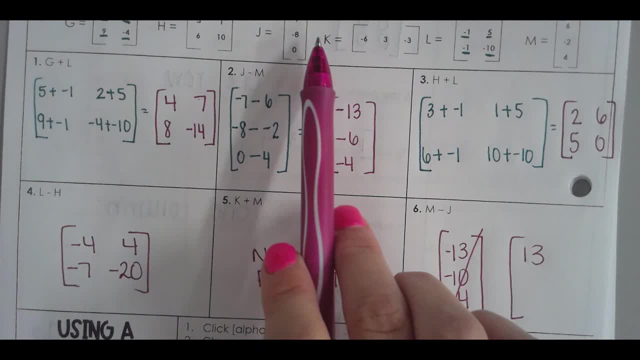 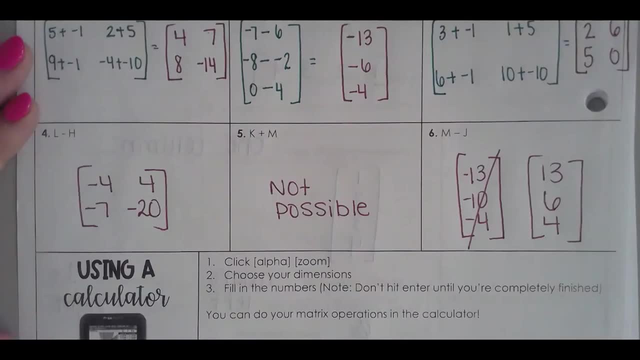 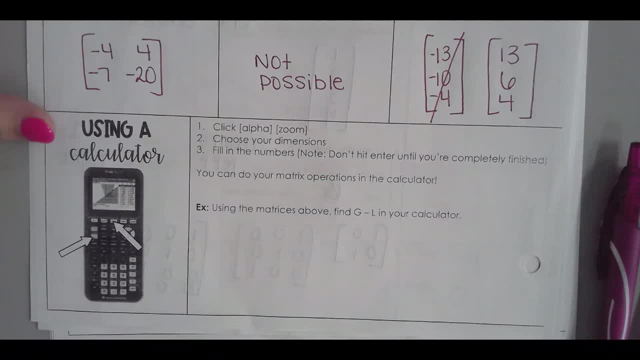 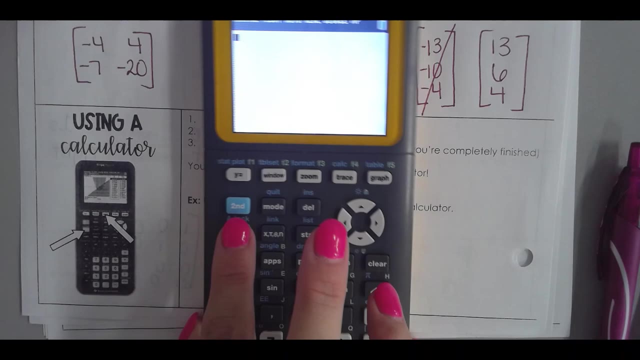 However, it's going to take longer to type it into the calculator. It would just add and subtract, But I'm still going to show you All right. So the easiest way to do this is to just type it into the calculator. Hit the copy button. 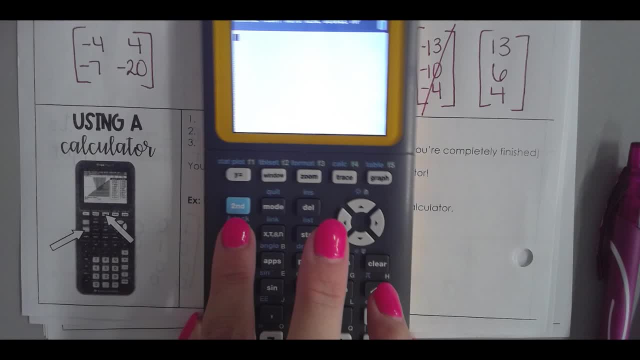 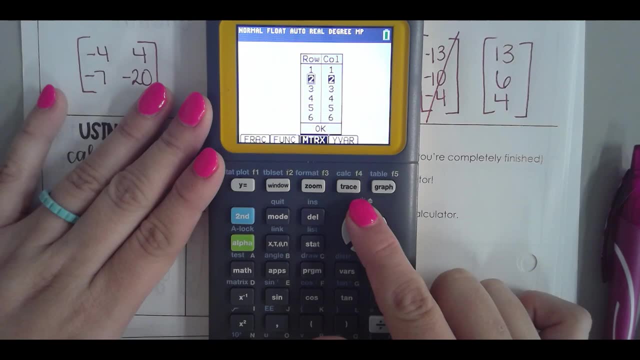 Zoom, Click up, Click on the drinking water. Note, after checked the calculator, Click on select And click on change. It'll show you it about 25 times. Thank you. It sets our calendar. see the categories, and from now we'll just find this one. 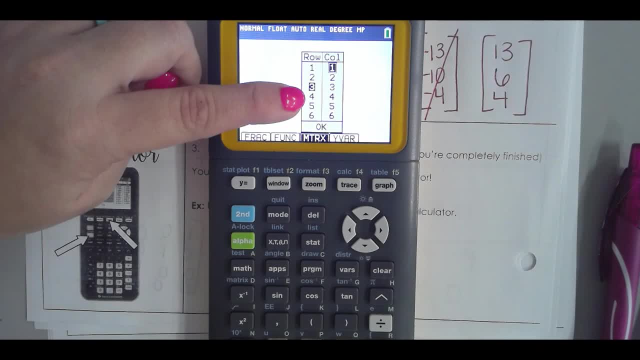 So those of you that don't know what you need for this week, you need to go to the description of this video. I've listed in the description the three columns I'm going to link, If you're excited to try something. fun videos. I'd really like the top. 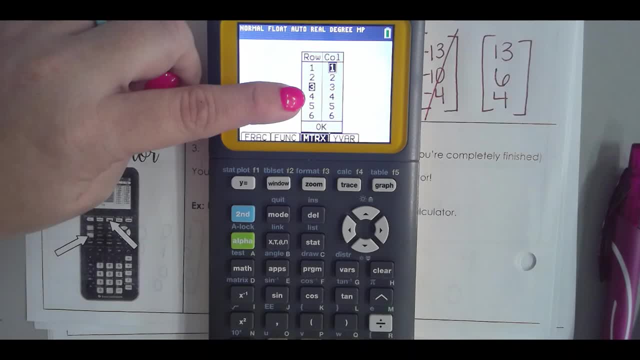 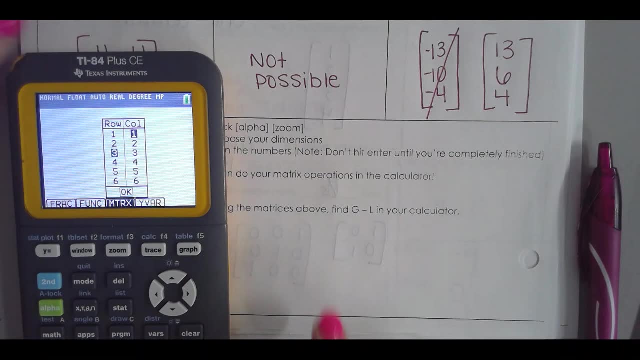 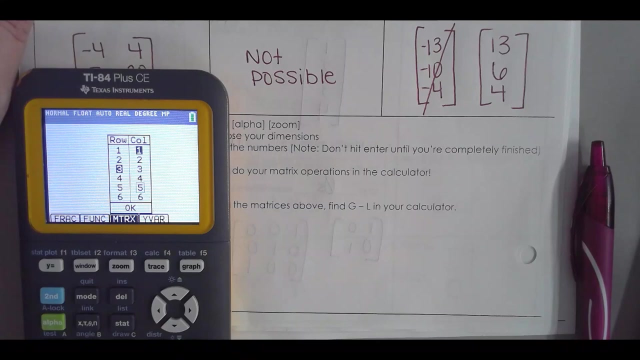 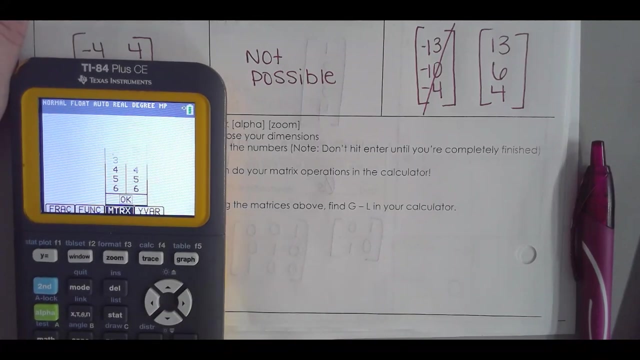 zoom and then, when you have the dimension selected, you go back down to okay and you just asking: is G minus L2s? so I actually want to do two by twos. so I'm gonna go two by two, hit okay, and then I'm gonna type in matrix G. 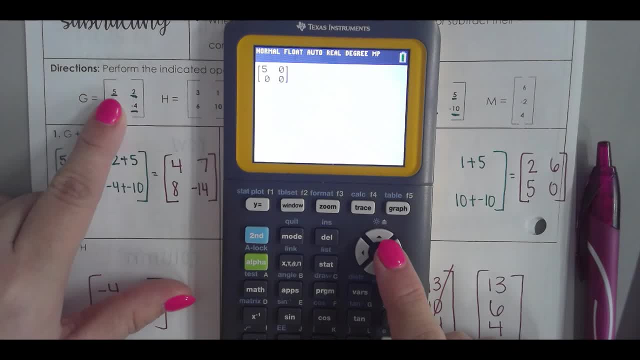 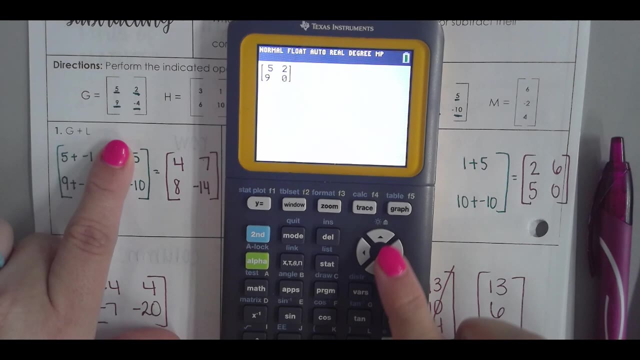 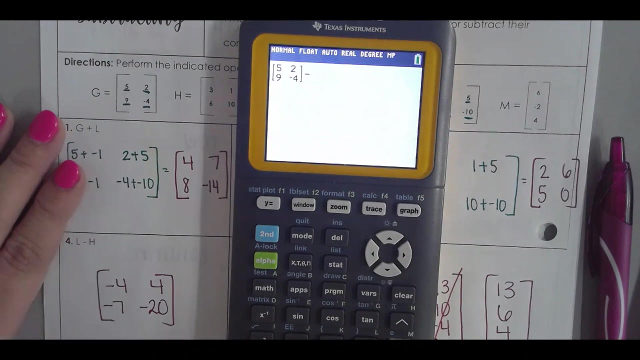 the right arrow, type in the two: if you hit the bottom like you don't have to have, you don't have to hit down and left if you just keep hitting the arrow, right arrow, negative four minus. so I'm gonna go outside minus and then type in the